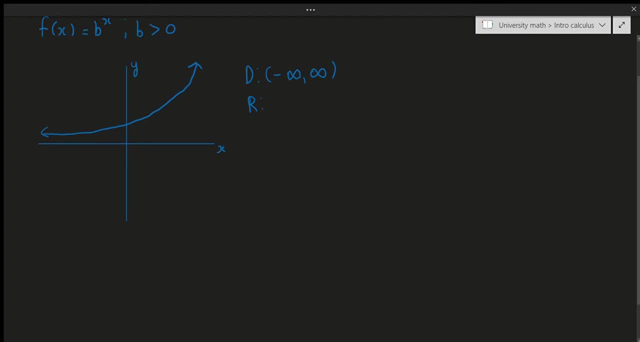 it can never actually read zero. For it to read zero, the x value has to be minus infinity. and because we can never actually reach minus infinity, the range of this function. well, the lowest value is going to be 0, and the highest value is infinity, none of which we can actually. 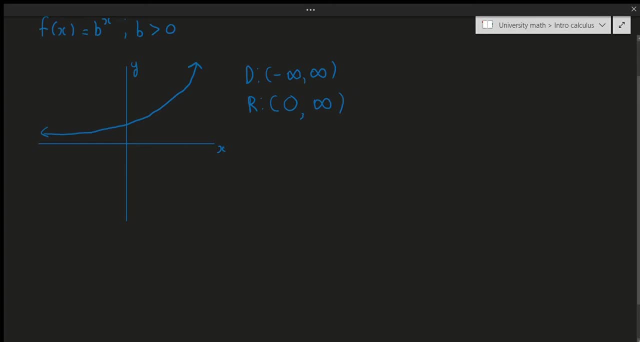 reach, of course. So that is what exponential function essentially looks like. Okay, so let's go in and talk about the rules of exponential functions. So remember that the exponential function is essentially something that looks like that. So let's talk about some rules, So rules. 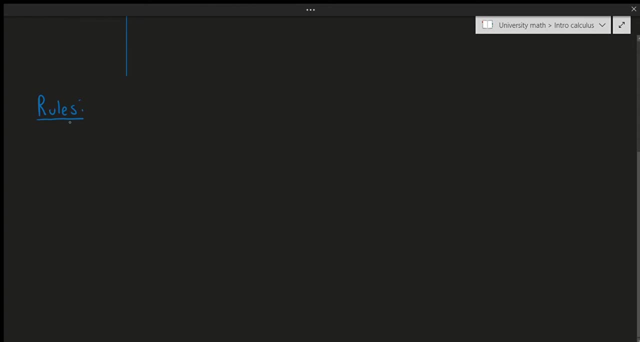 Okay. so the first rule is: if I have b to the power of x plus y, this is equal to b to the x times b to the y. So nothing too complicated. The next one is if I have b to the power of x, 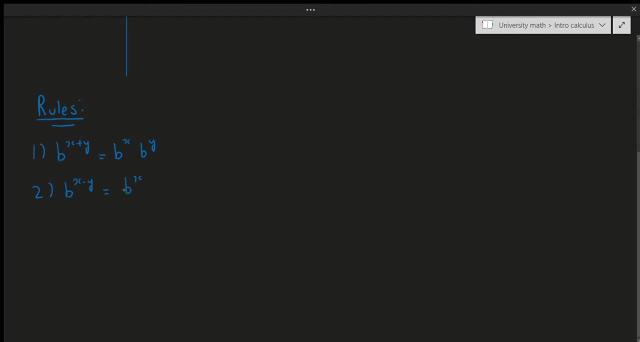 minus y. this is equal to b to the x divided by b to the y. So once again, nothing too clever. The next one is: if I have b to the x times y, So both of these are exponents. I can simply take the two exponents and multiply them. 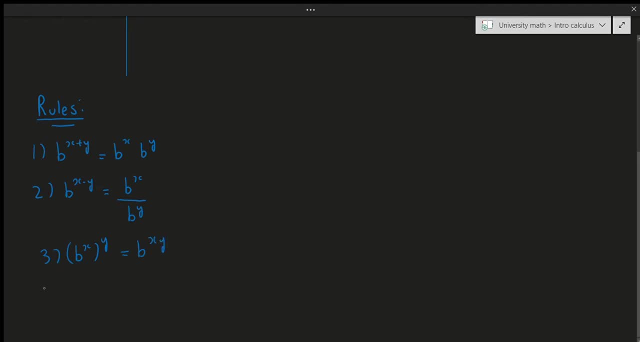 together. So we get b to the x times y. The last one is: if I have a times b to the x, well, that's equal to a to the x, times b to the x. Okay, so that's not too bad so far. 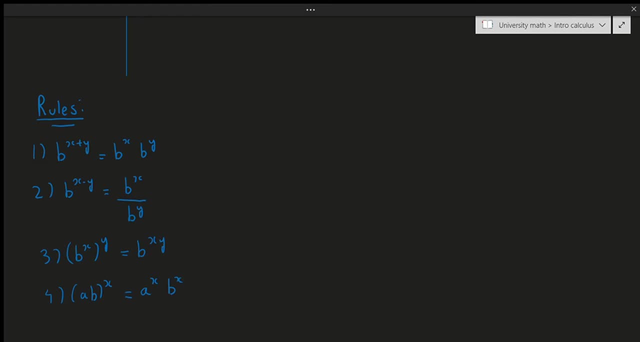 The next one we have to talk about is what happens when we have radius of x times y. So if I have a times b to the x, well, that's equal to a times b to the x, something to the power of zero. So what is b to the power of zero? 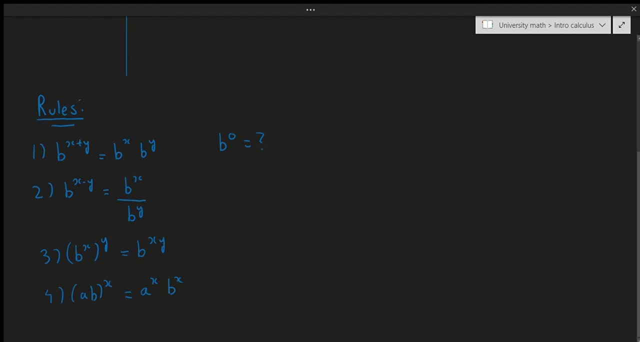 Now, from high school, or maybe a little bit earlier, you might have learned that's equal to one. But why is that? Why is anything to the power of zero one? The following is not really a proof, but more of a demonstration as to why b to the power of zero is one. So for this example, 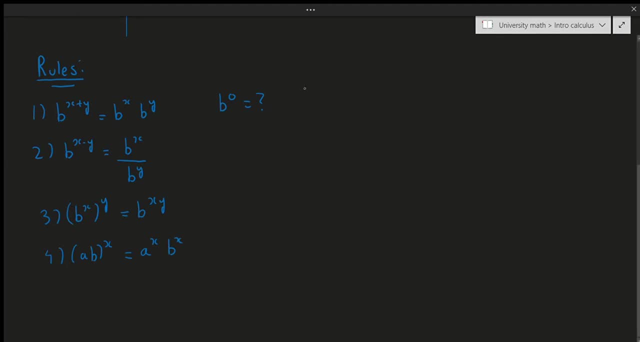 I'm going to use 2 to the x for no particular reason. This will work for any situation, So let's talk about 2 to the x. for a second. Well, suppose I calculate several values of 2 to the x, So let's say I start with zero. 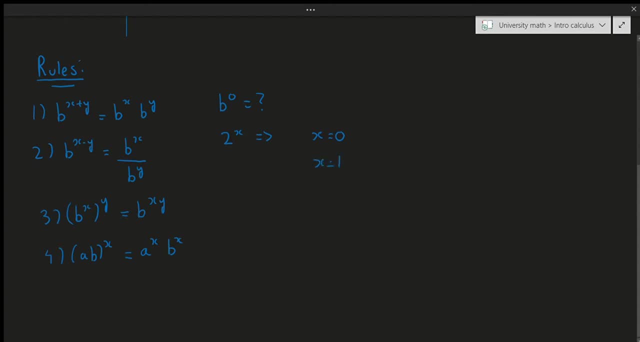 which, of course, we're trying to find. So then, we start with x equals 1,, x equals 2,, x equals 3,, x equals 4, and x equals 5.. Okay, so, 2 to the 5,, 2 to the 4,, 2 to the 3,, 2 to the 2,. 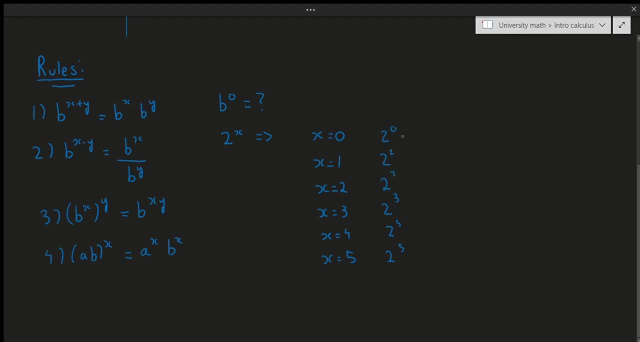 2 to the 1, and 2 to the 0, which of course we're trying to calculate. So let's go ahead and calculate these values out. So 2 to the 5 is 32.. That's 16.. That's 8.. That's 4.. That's sorry, that should be a 1.. This is going to be 2.. And 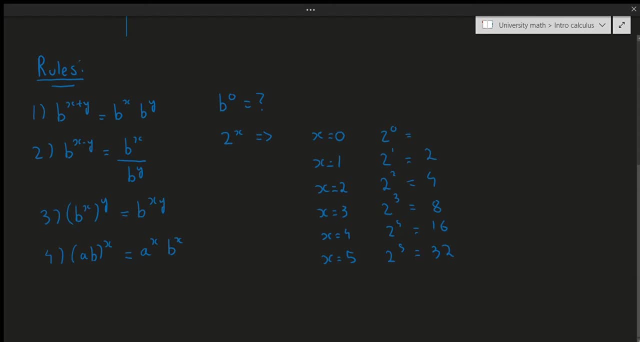 this one? well, we don't know. So what did we do? Remember what 2 to the x really is. 2 to the x is just essentially saying 2 times, 2 times, 2 times 2.. Then we just keep going x number of times. So this would be x times, So nothing too unusual. so. 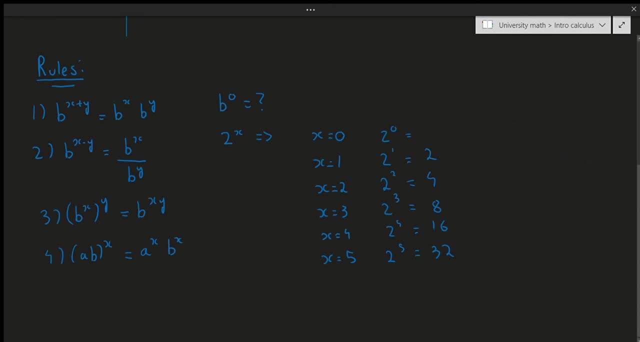 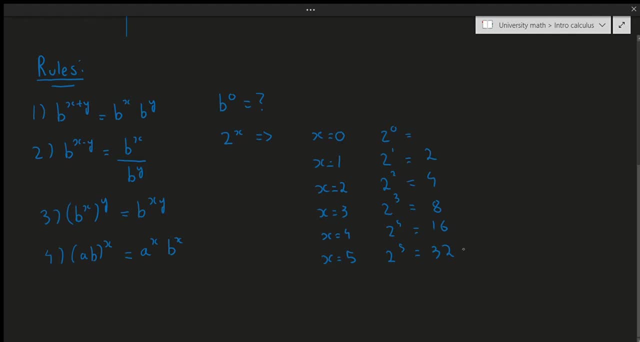 like 5 times. But notice that if I divide 30, 32 by 2, I get 16.. 16 divided by 2 is 8.. 8 divided by 2, that's 4.. I can do the same thing. 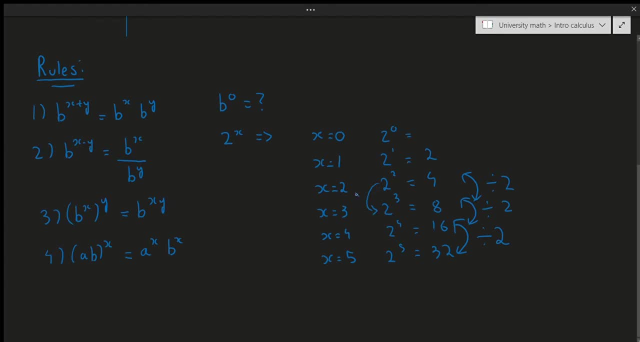 by going the other direction. So, for example, 4 times 2, that's 8.. 8 times 2, that's 16.. 16 times 2, that's 32.. And so on and so on. So we can always divide to, we can always divide to go. 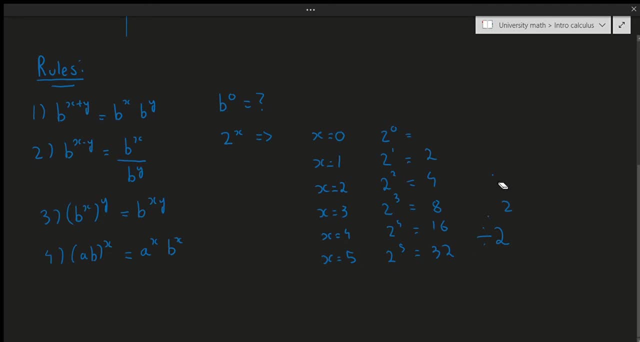 backwards. So let's use this strategy and kind of go backwards. So 32 divided by 2, 16.. 16 divided by 2, 8.. 8 divided by 2, 4.. 4 divided by 2, 2.. 2 divided by 2, 1.. So that means 2 to the power. 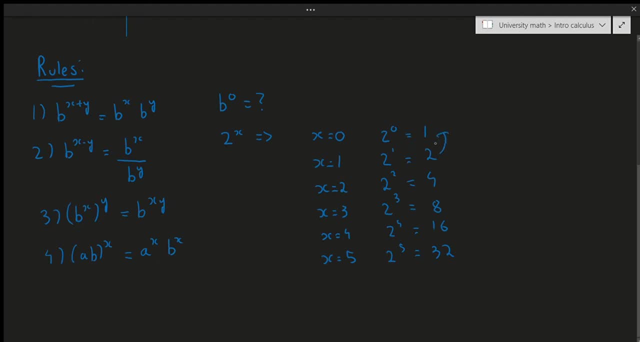 of 0 is 1.. And the reason for that is because 2 divided by 2 gives us 1, which is the same kind of patterning we use for the other situations. So, in general, b to the power of 0 is always. 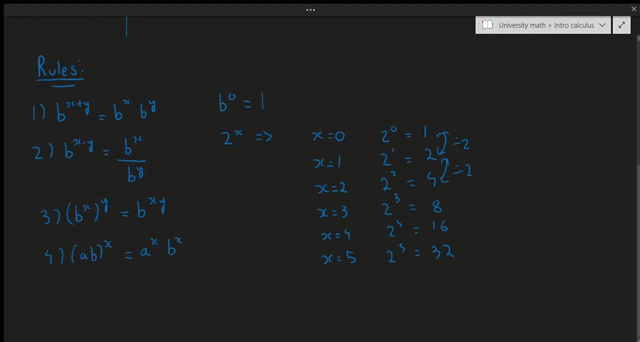 equal to 1.. So hopefully that makes a bit more sense as to why anything to the power of 0 is 1.. Okay, So with that out of the way, let's talk about something called Euler's constant, or sometimes whether that's people call it Euler's constant, but the proper pronunciation. 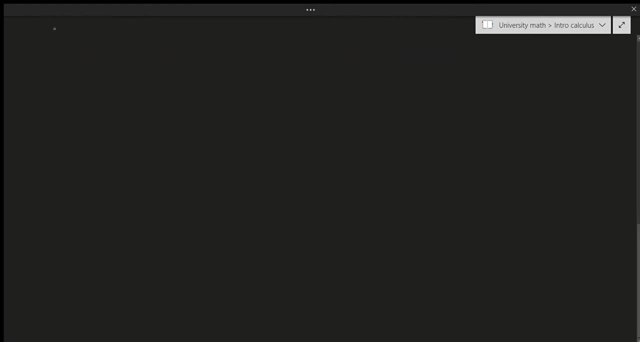 for this would be Euler's constant. So let's talk about this. So Euler's constant, So kind of like what pi equals 3.14159, and so on, there is something called Euler's constant which is: 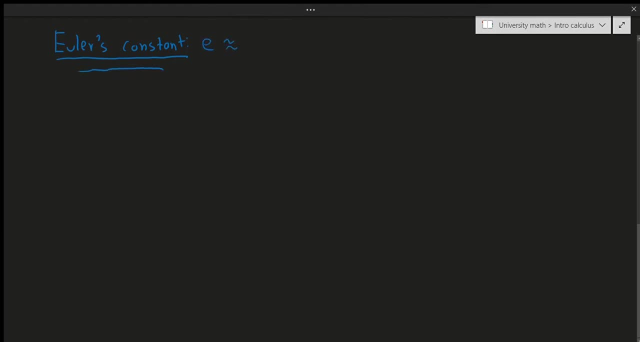 the constant E. So E is approximately equal to 2.718,. I believe, Yeah, 2.718.. And so on. Now, how is this derived? Because pi, for example, is the ratio between the circumference of a circle and its diameter of a circle, or radius 1.. 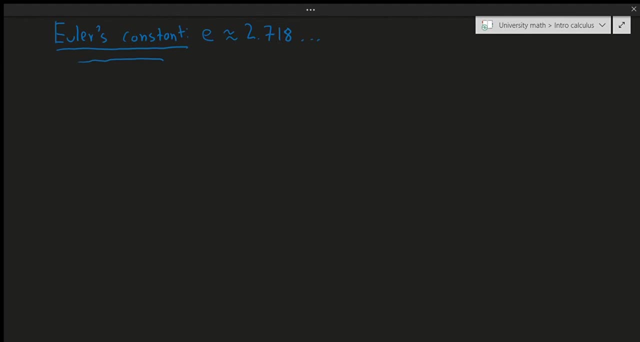 How does it work with E? How does that work? So for this one we have to look at a bit of history and talk about compound interest. So suppose I tell you that the amount accumulated for an initial amount of money called the principal is equal to p times 1 plus the 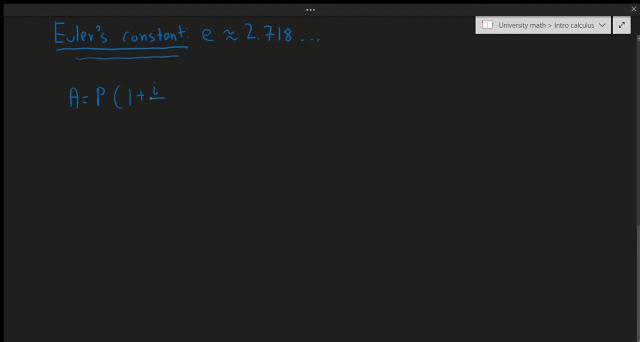 interest rate divided by n to the power of n, So the number of compounding periods, So semi-annually, annually, and things like that. So this is something that you should have covered in high school, but essentially, compound interest is basically done with this formula. So 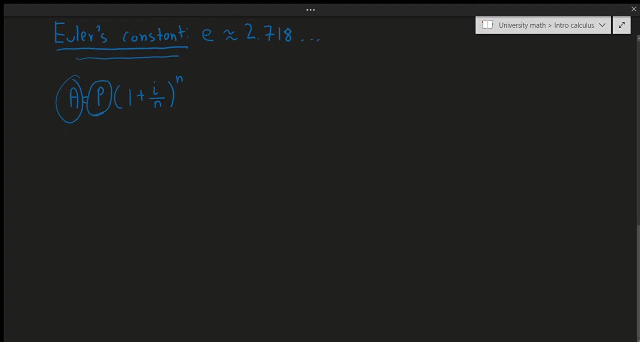 the amount accumulated for some principal out of money is equal to p times 1, plus the interest rate divided by the number of compounding periods, to the power of the number of compounding periods, which in this case is n. Okay, So suppose I tell you p equals $1. And suppose the interest rate is 100%. This 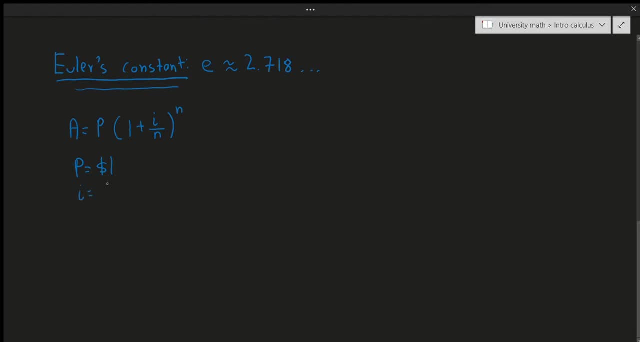 would never happen in real life, but let's just pretend it is. And typically, because i is given as a percentage, I'm just going to pick 1, which is the same thing as 100%. Now suppose I tell you that n equals 1.. Okay, Well, that means we get 1 times 1 plus the 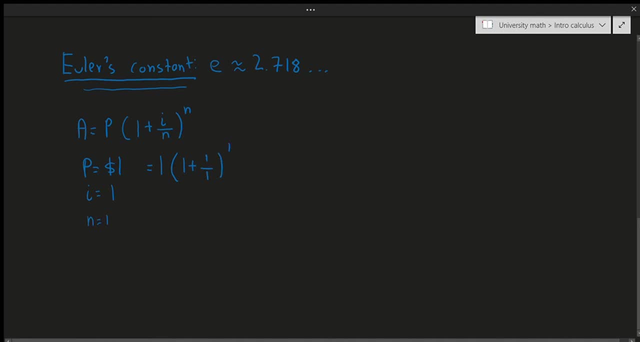 plus well, 1 over 1 to the power of 1.. So that's going to give me 2.. Okay, What if I made this even more frequent? Notice that the more frequent I make my compounding periods, so the 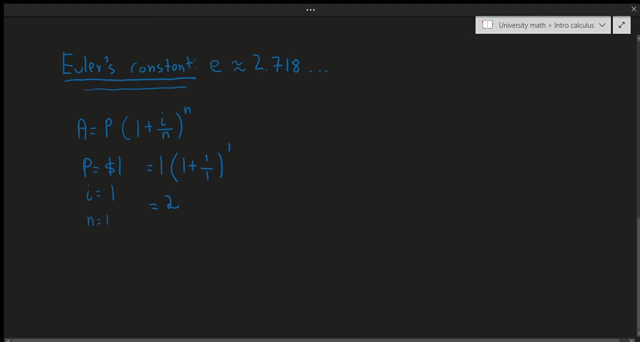 more frequent. n is the more amount of money I make. So suppose I tell you n equals 10, or n equals 100, or 1000, etc. Notice, the amount of money you make actually goes up. So for example, 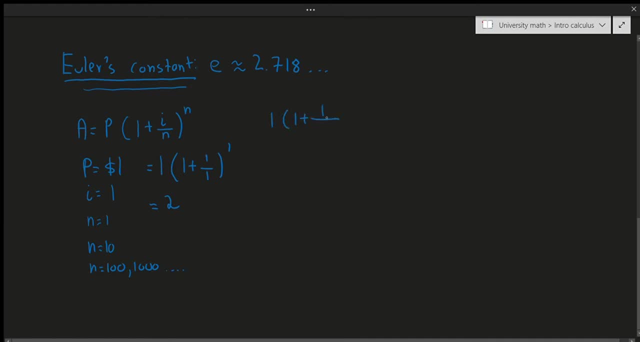 1 times 1 plus 1 over 100 to the power of 100 is a lot more than $2.. So this is a really big amount. So let's go ahead and actually calculate this amount, out of curiosity. So 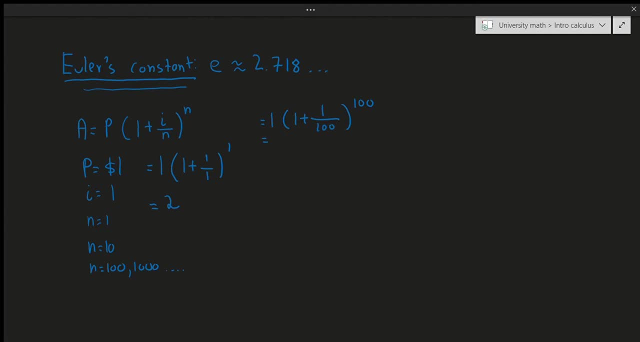 if you go ahead and calculate this, we obtain that, the principal amount. so let me just do this out real quickly. So 1 over 100 to the power of 100. So this amount is actually equal to 2. 7048.. That's very interesting. That's really close to this value. So what if we compounded? 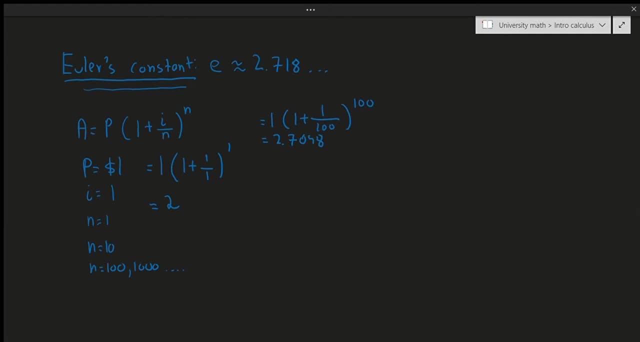 so frequently that we compounded an infinite amount of times. So that's very interesting. Now, technically you can't plug in infinity, but I'm just going to be a little bit liberal at this point of time. So let's go ahead and say: I have $1.. My interest rate is still. 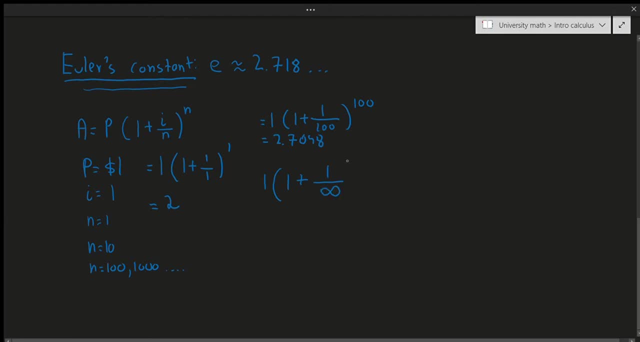 1. And let's suppose I compound an infinite number of times. You can't really do it. You should be doing a limit for this technically, but I'm going to be a bit liberal here. So if you go ahead and do this, you actually get the number E, which is well what we. 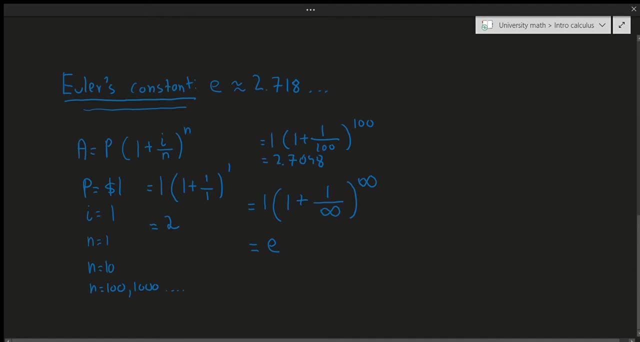 had before. So that's essentially how Euler's constant was discovered. Bankers kind of caved the way for this constant to be found And of course this came after Leonard Euler, who was one of the most famous Swiss mathematicians of his time. 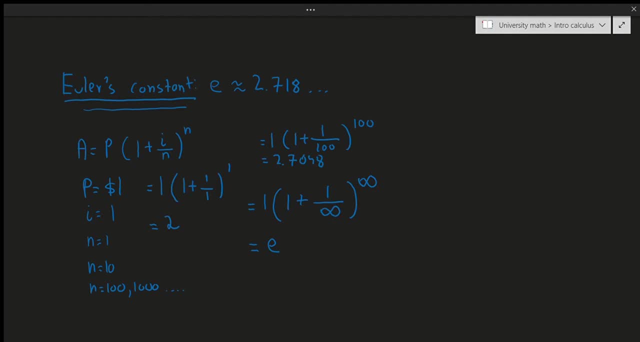 So that's essentially what Euler's constant is, And we will use this concept a lot in calculus and beyond, just because it's something that's used so often. So, with that being said, let's move on to the next topic, which would be logarithms. So let's go ahead and 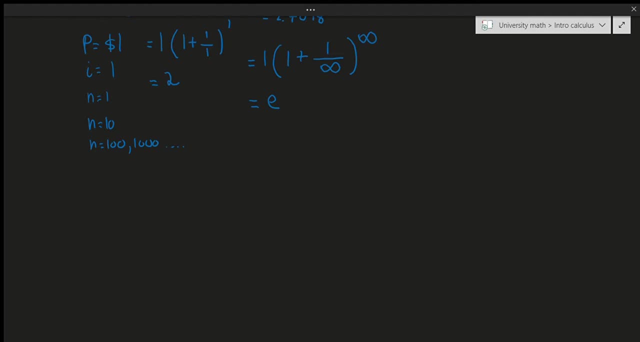 talk about what a logarithm is for a second. So a logarithm is essentially the inverse of an exponential function. So let's go ahead and write down the definition: So logarithm, Okay. So let's go ahead and write that down. Okay, So the logarithm. 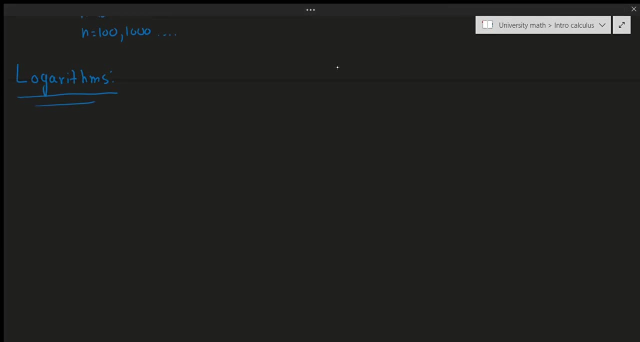 is the inverse of an exponential function. So to kind of remind you what an exponential function was, it was a function that essentially looked like this: So y equals b to the x, So of course, an inverse is a reflection about the line y equals x. 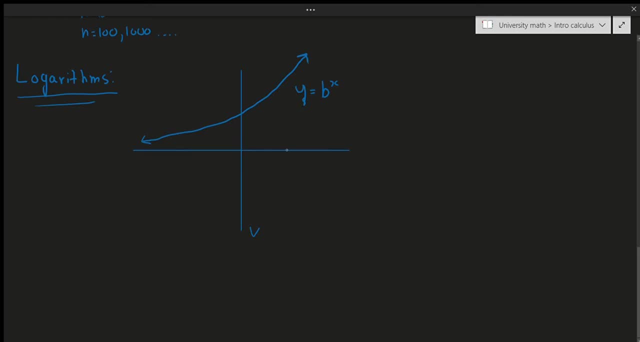 So a logarithm would look something like that. roughly So, the notation that we use for a logarithm is: well, we literally write the word log. So if y equals b to the x, the inverse of the logarithm. 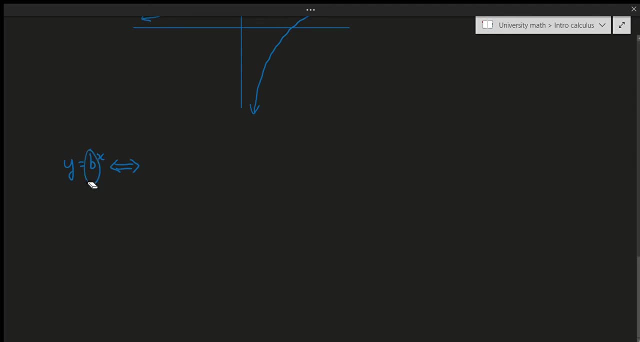 well, it depends on what base we use. So we use the word log base b because it depends on the base we're using. So log base b of y is equal to x. So this is essentially what a logarithm is. It is the inverse of an exponential function and it's how we use to solve for. 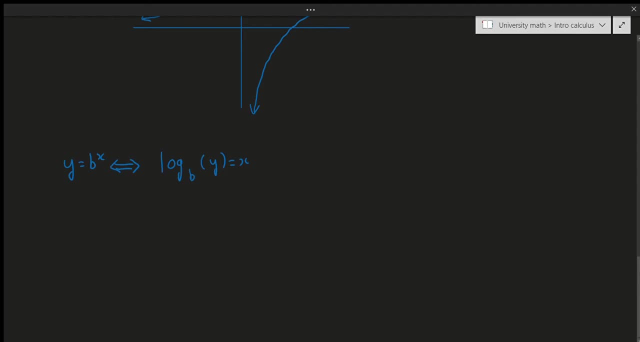 what x is. So, as a consequence, we can use the cancellation formula. So let's go ahead and talk about some properties, and talk about some properties of logarithmic functions. Excuse me, So let's go ahead and talk about some properties. Remember that. 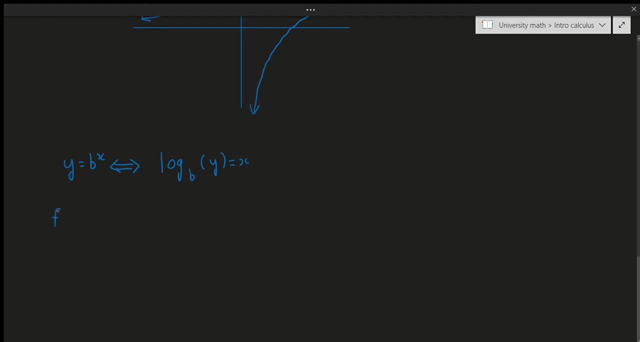 for the cancellation formulas we have that f inverse of f of x is equal to x, and we also know that f of f inverse of x is equal to x. So therefore we can get some nice properties from this. We know as a result, that log base b of b to the x is equal to x. So 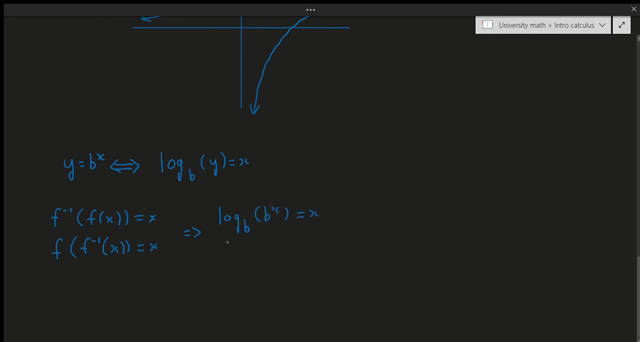 that's always equal to x. and we also know that b to the power of log base b of x, that's also equal to x, as a direct consequence of these cancellation formulas which we talked about in the last videos. Okay, So let's go ahead and keep going with this kind of. 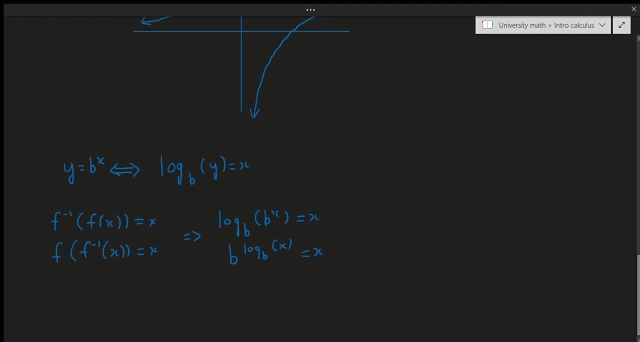 assumption. So, as I mentioned, the inverse of an exponential function is a logarithmic function. So the domain and range for a logarithmic function, this flips around. So if the domain for an exponential function was minus infinity to infinity and the range for an exponential function was from zero to infinity, this flips. 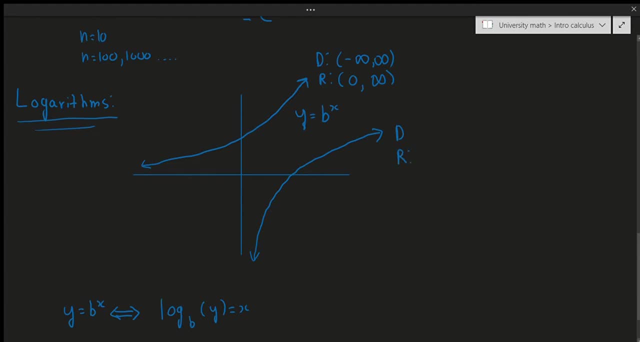 So for the domain of a logarithmic function the domain would be from zero to infinity and the range would be from minus infinity to infinity. And that should kind of make sense. just by looking at the graph You can see it can go down. 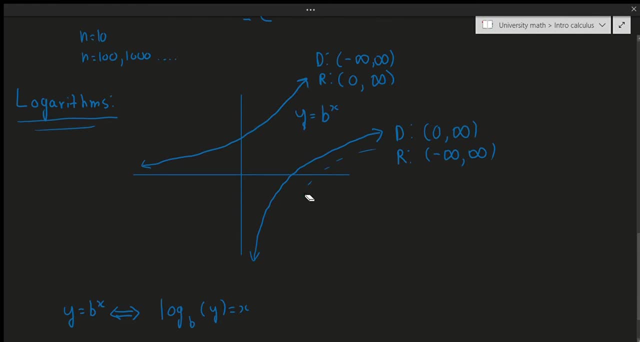 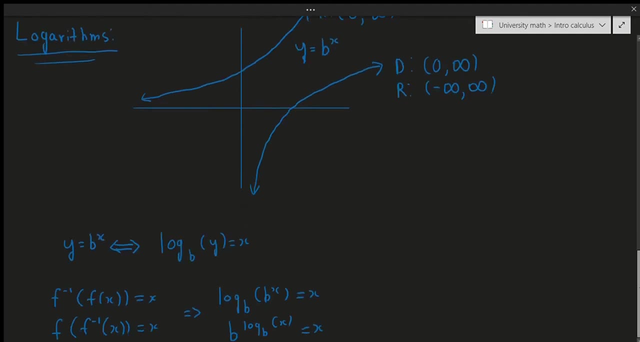 You can see it can go up forever and then you can keep going up forever. So the range is from minus infinity to infinity, and domain it has to be at least zero or more. So that's kind of how this works. So nothing too bad so far. Okay. So the next thing we can talk. 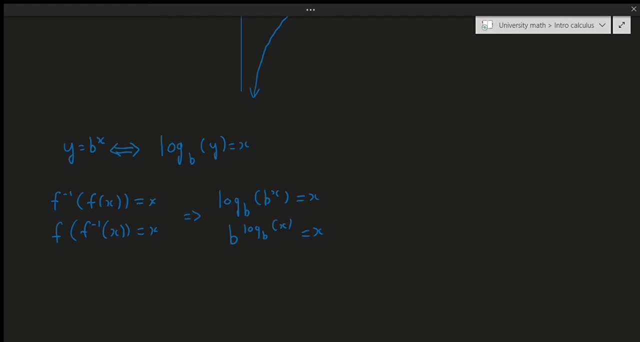 about is the laws of logarithms. The laws of logarithms are very similar to the exponential laws we were talking about earlier. So these laws, except there's a little bit more of them, And there's one important formula that we're going to talk about in a little bit. 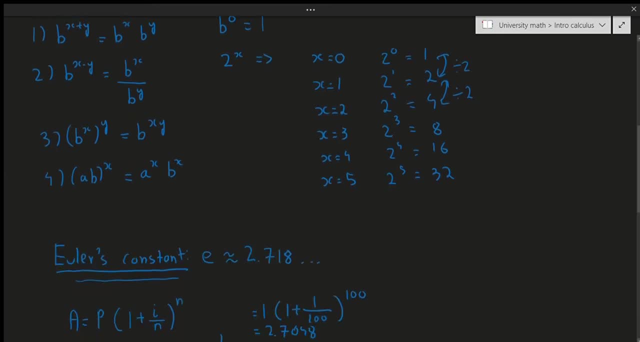 There's a formula which we have to talk about in a separate kind of section. So let's go ahead and get right to it. So we can now talk about the laws of logarithms. So let's go ahead and talk about that. So the laws of logarithms, Okay. So let me just underline: 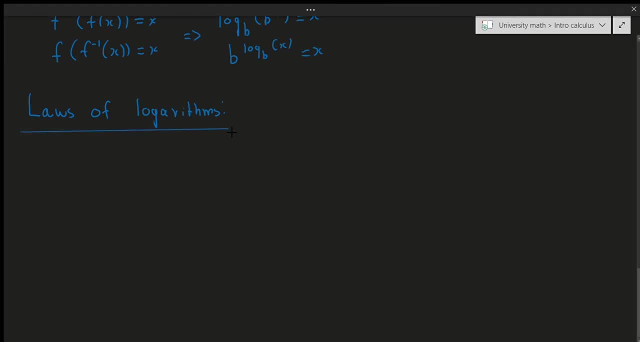 this. Okay. So the first law is that the log of x times y for some base. it doesn't matter which base we have, this is always equal to log base b of x plus log base b of y. Okay, So the next one: if we have log base b of x over, 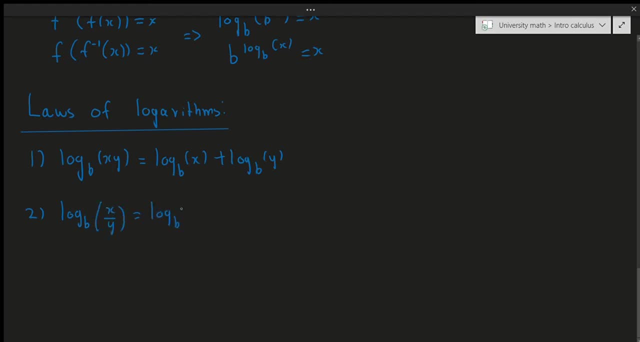 y, this is equal to log base b of x minus log base b of y. So again, nothing too crazy so far. The next one is: if I have the log base b of x to the power of r, this is equal to r log base b of x, And we are assuming here that r is a real number, So r is in. 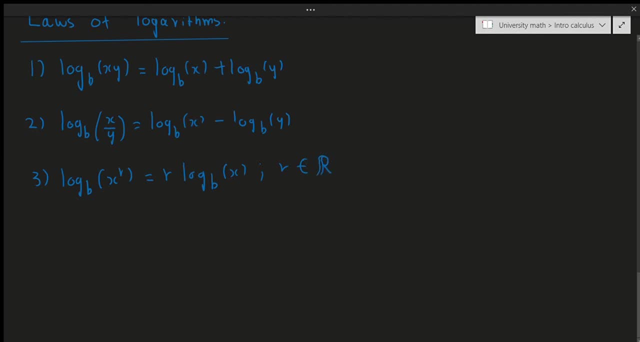 the real numbers. Okay, So there's nothing too crazy about that. So those are most of the basic laws you have to be aware of. There's something called the change of base formula, which we'll talk about a little bit later. So let's do some very quick examples just to kind of get that out of the way. So 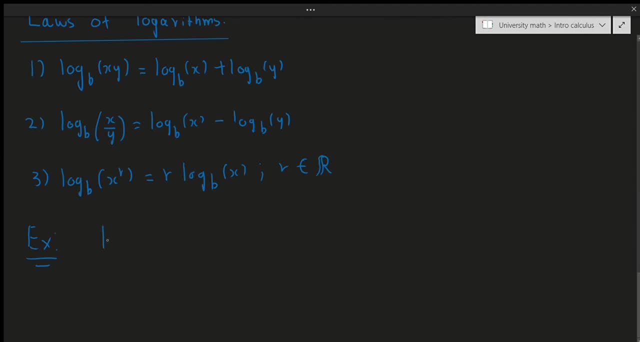 suppose I want to compute log base 2 of 80 minus log base 2 of 5.. Okay, This one is very simple. We can't do this individually, just because evaluating log base 2 of 80 is well, it can't be done. 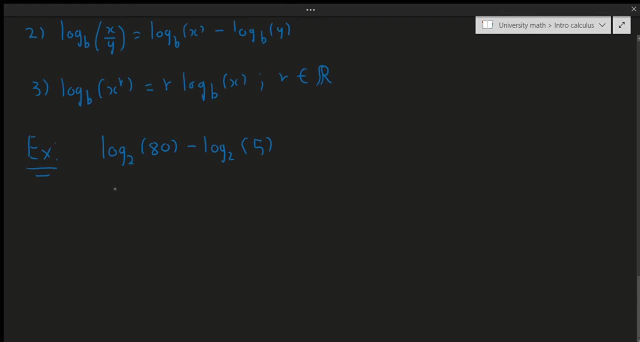 So, for example, if I wanted to do this individually, we would have to do it like this. So log base 2 of 80, we have to make sure we have to let that equal to x or something, And then 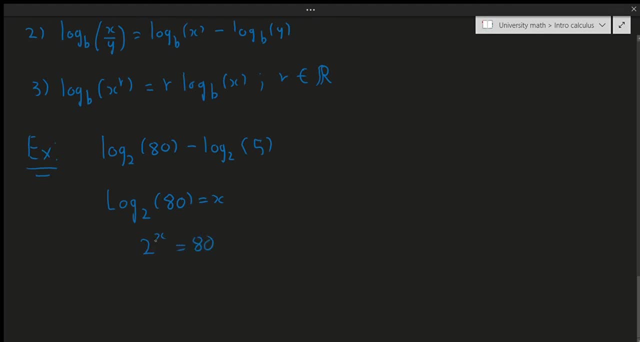 2 to the x has to be equal to 80. So you would need to find an x value such that we got 80. But unfortunately, well, there's no such number. well, no nice number at least. So as a result, we've got to do this a little bit differently. 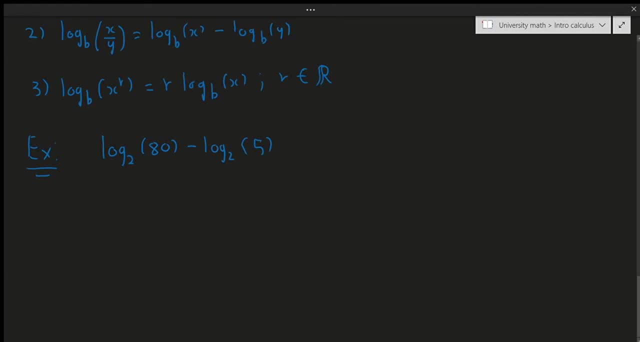 Let's do that right now. So if you want to do this individually, you can use the second law of logarithm. So we're allowed to write this as log base 2 of 80 divided by 5. That gives us log base 2 of 16.. We're not quite done yet, because we can now use this property. 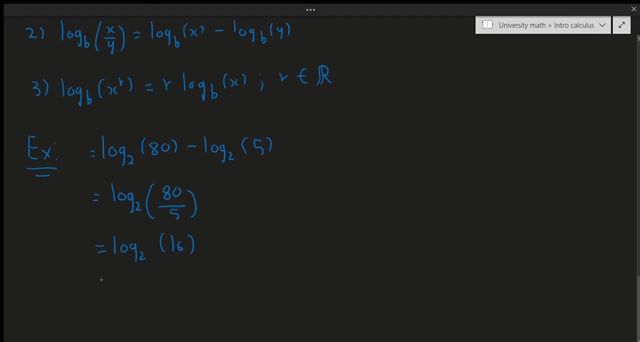 right there. Not yet, but we will be able to soon. So right here we can write this as log base 2 of 2 to the 4. because 2 to the 4 is 16.. The 4 can now be taken out, So we can write this as 4 times log base 2. 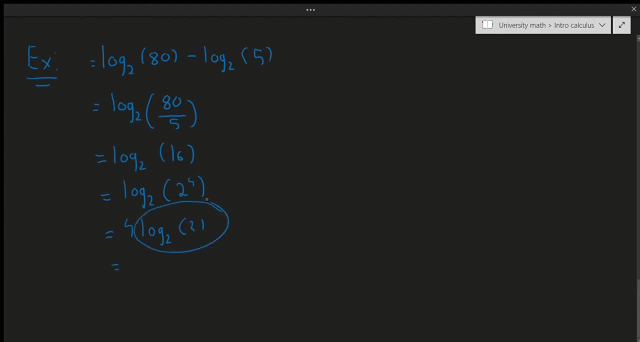 of 2.. But of course this right there is equal to 1 because of the cancellation formulas. So we get 4 times 1, or 4.. So not too complicated. We just have to be a little bit careful about the. 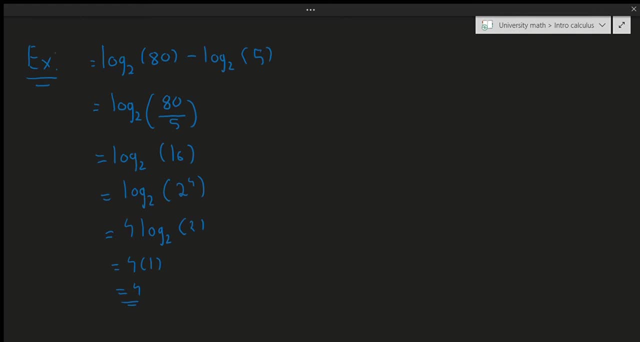 laws of logarithms, But otherwise not too bad. So let's go ahead and talk about what a natural logarithm is, So that one is a little bit harder to contact, but still not too bad. Okay now, earlier I mentioned for that, for a logarithm, the base of the logarithm is kind of 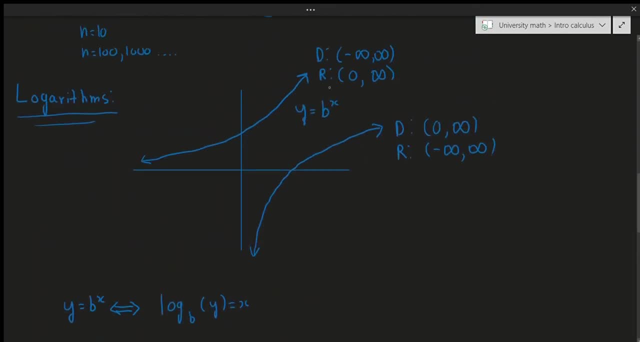 determined depending on the exponential we're working with. So if I have y equals b to the x. the inverse would just be log base b, So so the base depends on the original exponent that we were working with. So earlier we talked about e, So let's go ahead and use that in this kind of concept here. So any logarithm with a base of e. 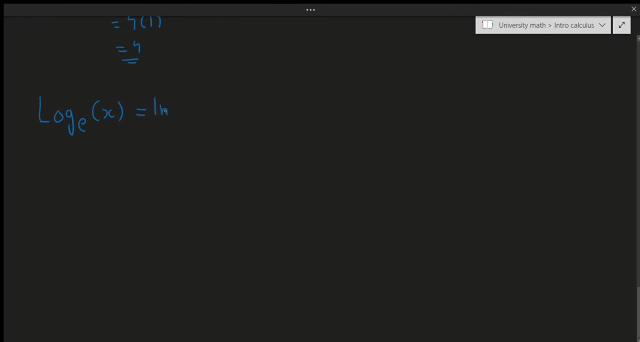 is called the natural logarithm of x, And sometimes this pronounces ln of x. This logarithm is used so often. we just call it a shorthand notation. So we use the letters ln and n, So ln of x. So once again, log base e of x is used so often, it's just often abbreviated. 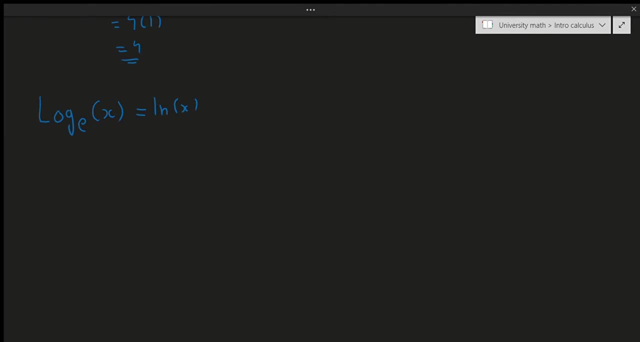 as ln of x. There's nothing crazy about this. We just have to remember that this is the same as log of x with base e. So nothing too crazy so far. So the same rules that we were talking about earlier still hold. There's nothing different about them. So the rules are still exactly the same. 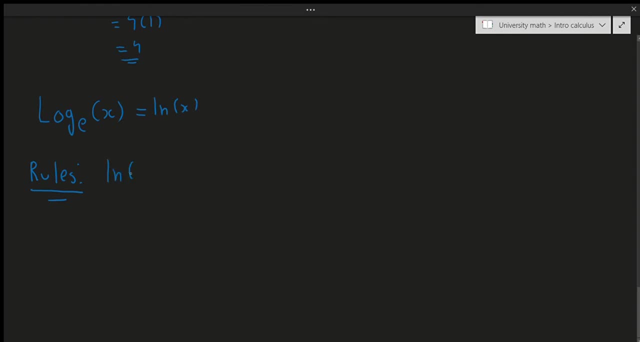 So, for example, ln of x. if this is equal to y, that means e to the y equals x, And the reason for that is because, once again, the natural logarithm of x is equal to log base e of x. So e to the power of y is equal to x. 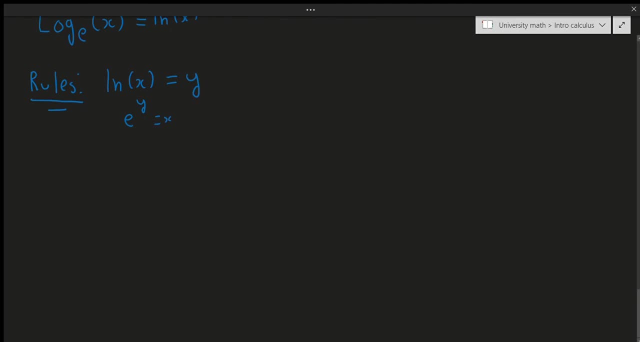 so that's the first rule. The other rules again, there's nothing. there's no major difference between a natural logarithm and a logarithm. so the second rule. so this is the first rule. The second one is: the natural log of e to the x is just equal to x, and e to the ln of x is equal. 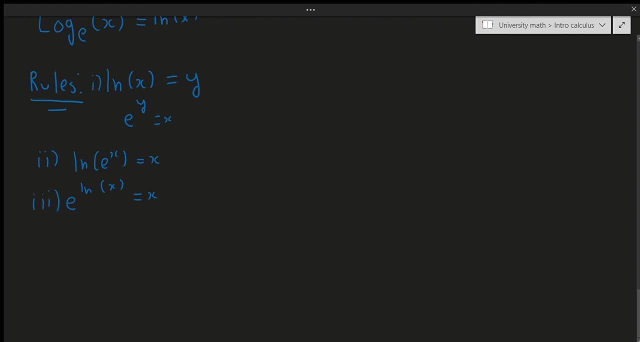 to x. so these are just a direct consequence of the cancellation formulas. Okay, so nothing too wild so far. Next one is: the natural log of x times y is equal to the natural log of x plus the natural log of y. so again, nothing too crazy so far. The next one is, if I have, 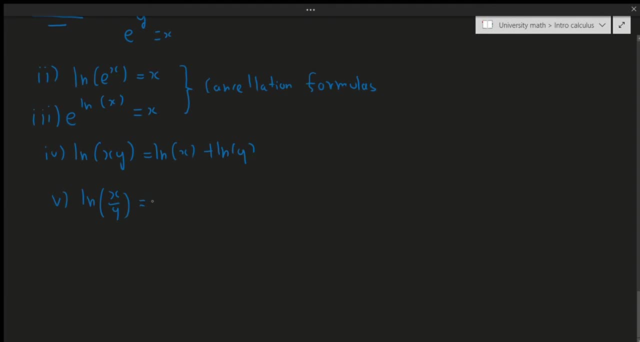 the natural log of x over y. well, that's equal to the natural log of x minus the natural log of y. so nothing too bad. The next one: it's the same as the other rule. so if I have the natural log of x to the r, that's equal to r natural log of x. I will use natural. 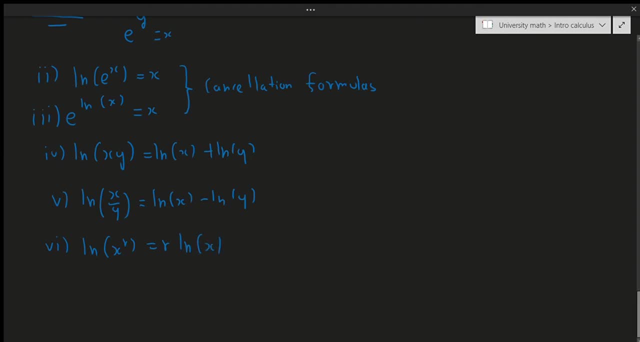 log ln and ln interchangeably they're the same thing. So the next one, so rule 7, so if I use the rule, if I use this rule right here, if I use the second rule, that would mean that if I have ln of e to the x equals x. that 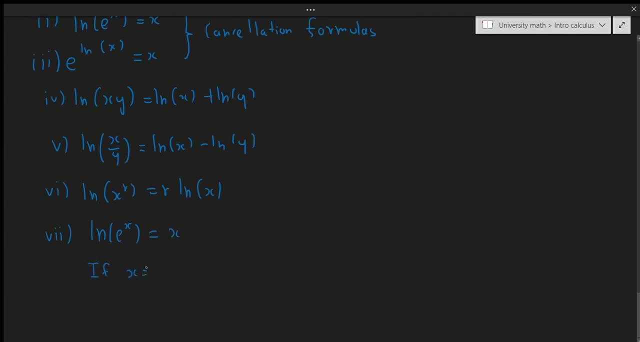 would mean that if x equals 1. we get that ln of e equals well, 1.. This one is actually really important. We'll use that quite often for later concepts, but that's another important one. So let's do a kind of. 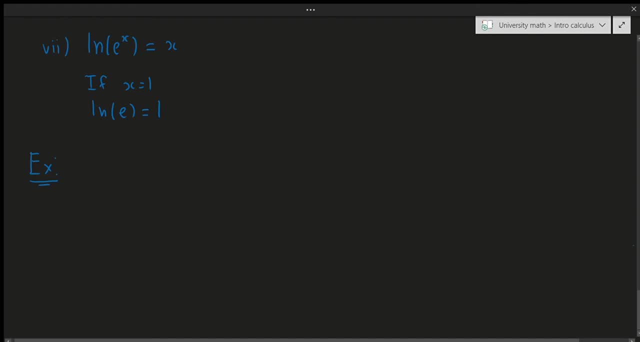 very trivial and quick example. So this is not supposed to be a very hard question, but this is just a taste of how to solve a natural logarithm. So if I have ln of x equals 5, that means, for example, x would be equal to e to the power of 5.. So nothing too wild about this. 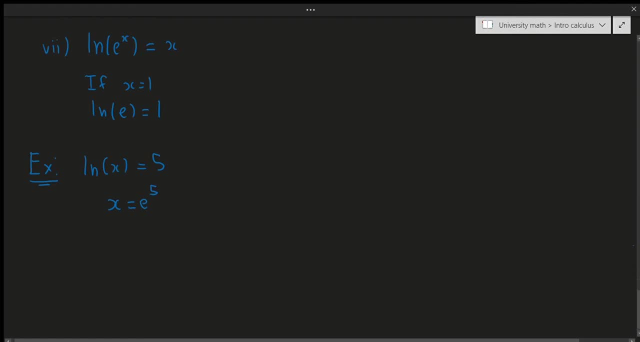 And because a natural logarithm is the same as a logarithm, it has the same domain and range of a normal logarithm. So the domain of a natural log would be from 0 to infinity and the range of a natural logarithm would be from minus infinity to infinity. 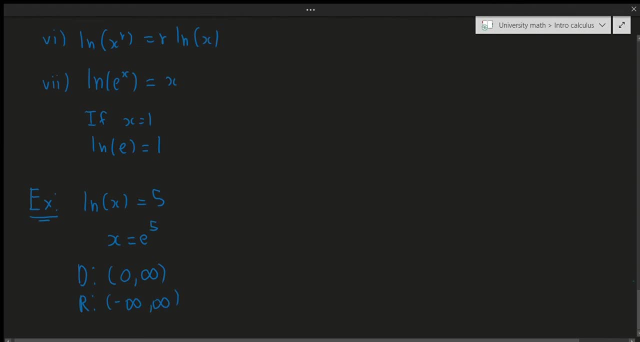 So nothing too crazy. So it's the same as a natural logarithm. it just has a base of e, So nothing too crazy. The next example, So this one: suppose we have e to the power of 5 minus 3x equals 10. And say we want to solve for. 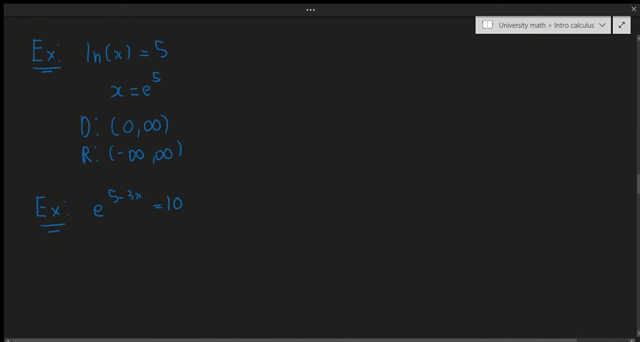 x. How do we do that? Well, kind of like in algebra, how you could take the square root of both sides, or you could square both sides, or things like that. We can just take the natural log of both sides. So what do I mean by that? I literally mean that we can go natural log. 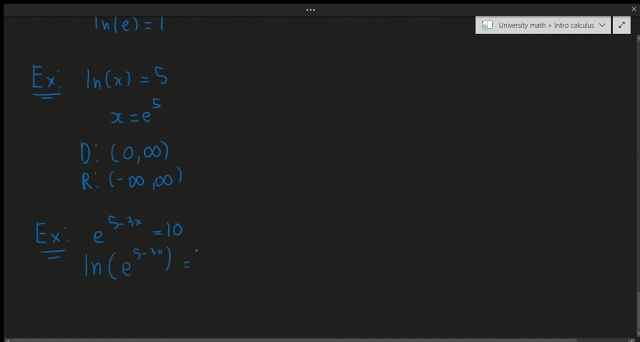 of e to the power of 5 minus 3x is equal to the natural log of 10.. This is fine, Like, for example, if I have x equals- I don't know, this is a very silly example. This is the same thing as the. 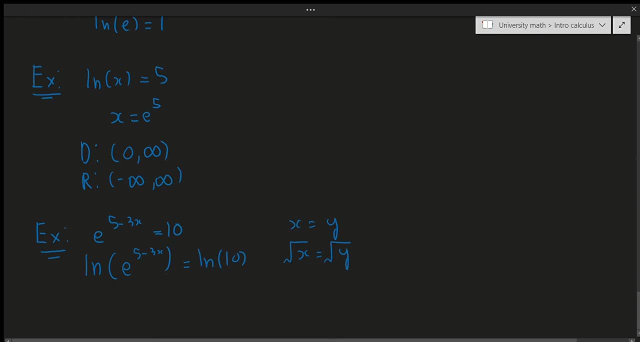 square root of x equals the square root of y, Like this is fine. So I'm allowed to do the same thing on both sides, as long as I apply it properly. So if I have an expression I can, or rather an equation, I suppose I can take the natural log of both sides. That's totally okay. 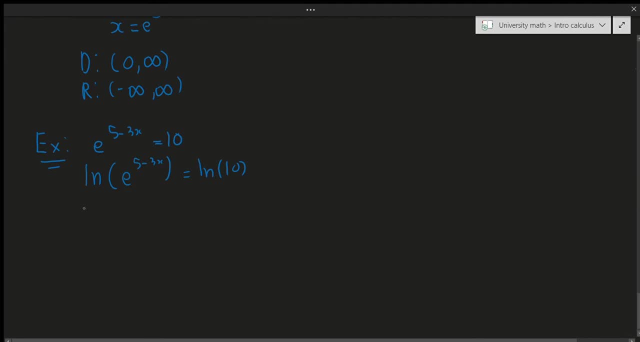 So now, using our rules for natural logarithms, we can pull the 5 minus 3x out, So we get the ln of e, And that's equal to ln of 10.. And then we can use the fact that ln of e equals 1.. 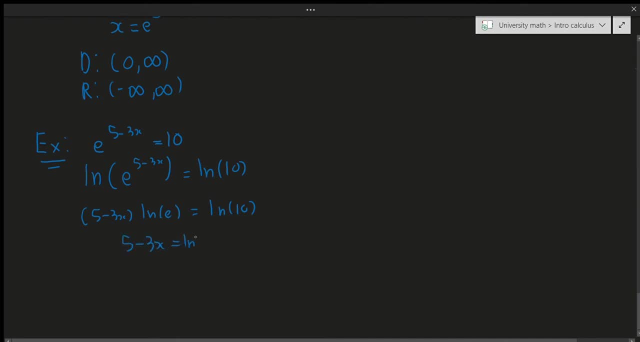 So we get: 5 minus 3x equals ln of 10.. And then we can go ahead and simply solve for x: 5 minus ln of 10 equals 3x. And then, if we divide both sides by 3, we get 1 over 3 times. 5 minus ln of 10 equals x, And that's it. Nothing too crazy there. 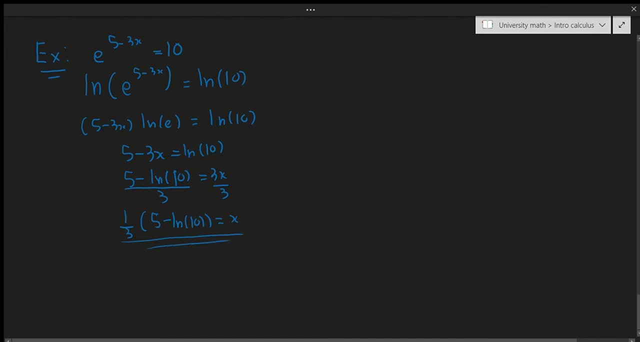 The last thing. I suppose there's two other topics. The last thing we have to talk about is the change of base formula. So let's talk about the change of base, Okay. So remember that, for a logarithm, we always have a certain base that we work with And the 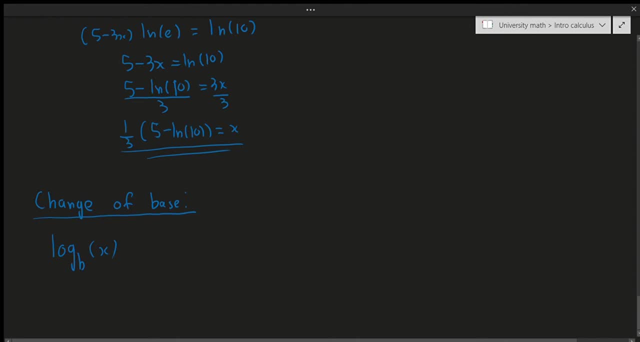 base depended on the exponent that we took the inverse of. So, for example, if we had 5 to the x, the base would be log base 5 of whatever is equal to x. So what if we don't like this base? Because, for example, computers use binary or base 2 notation But we use base 10 notation? 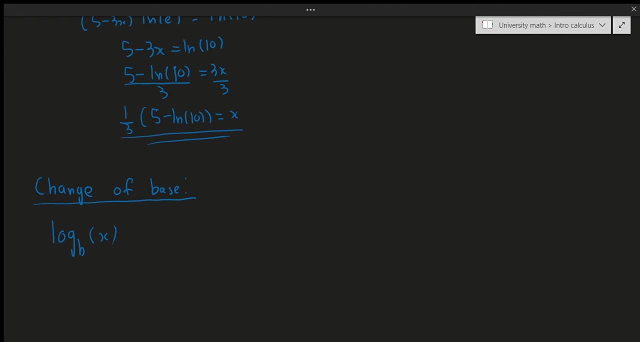 So there might be some times where you have to use base 16, notation or things like that. So how do you kind of change bases around? Well, there's a very simple way to do this. If I have log base b of x and suppose I don't like this base and I want to change it to another, 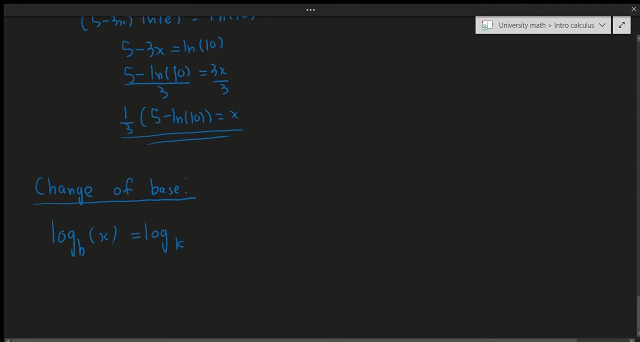 base k. So k is my new base of x divided by log base k of b. So sorry, there should be a b here. I wrote that really badly. Okay, So this is the change of base formula. The change of base formula. 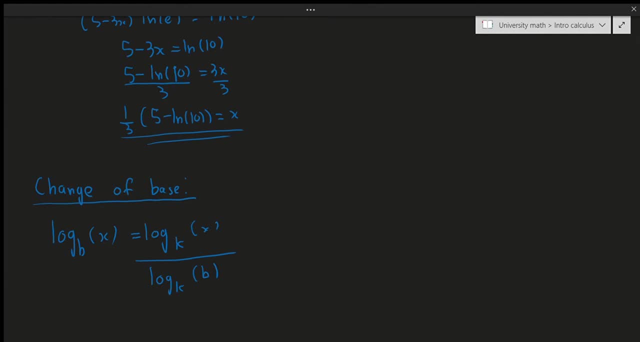 is simply saying that if I don't like the base I have, I can just simply change it around For a natural logarithm. it works the same way. So let's do kind of like a quick example of this, Although you wouldn't really use this with natural logarithms mostly. It's kind of uncommon, So we'll. 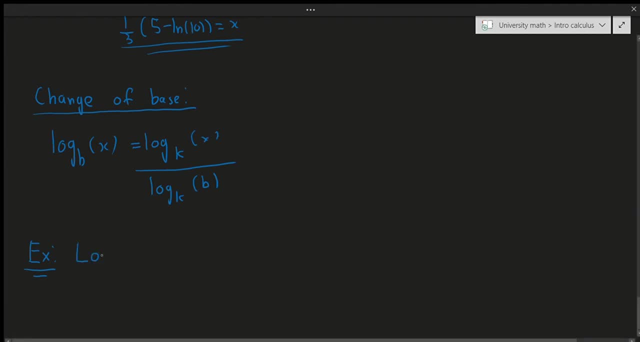 just take the normal logarithms. So suppose I have log base 8 of 5, and I want to change to base 10.. Okay, Well, that's equal to log base 10 of 5 divided by log base 10,. 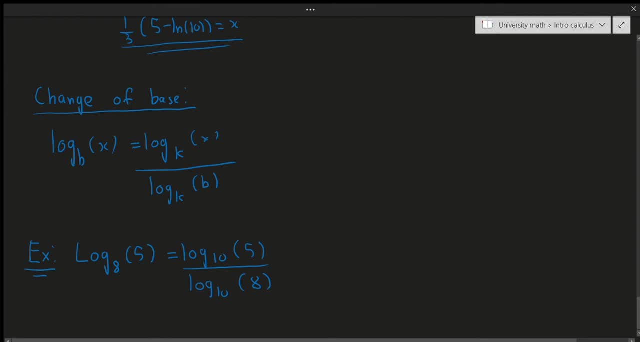 of 8.. So nothing too crazy And typically any logarithm written with base 10, the base can be ignored, So we can write this as log of 5 divided by log of 8.. So the reason we don't use a 10 for: 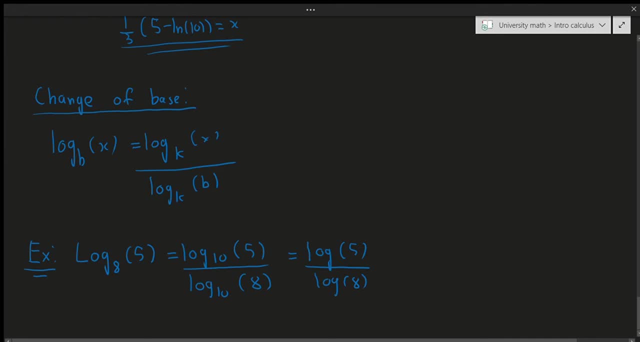 as a base typically is because it's used so often, we just give it a special name. This is usually called the common logarithm, just because it's used so often. So we can just usually drop the base. If there's no base in the logarithm, you can assume it's base 10.. So, for example, 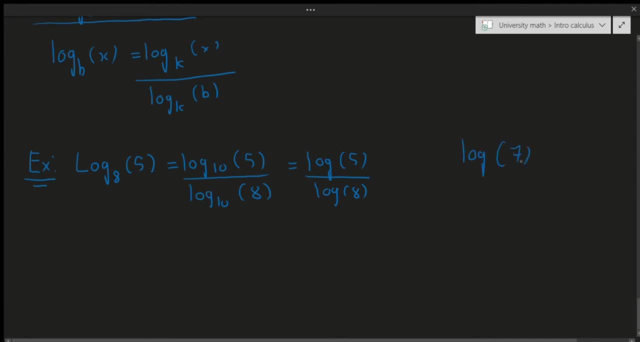 if I were to tell you log of- I don't know- 7,. this is the same thing as log base 10 of 7.. It's the same thing, Okay. So the last thing we should talk about in this video is graphing a logarithm. 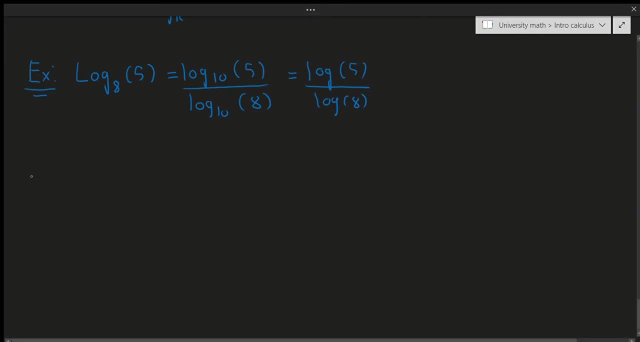 and transforming it. So suppose I wanted to graph the equation: y equals ln of x minus 2 minus 1.. And I'm asking you to plot this. Okay, So this one isn't so bad. So let's go ahead and draw a few axes. We will need at least three. 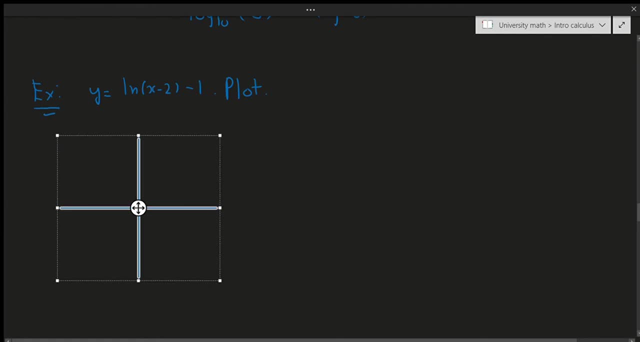 for this. So let's go ahead and draw them. So here's one, Here's the other And here's the other one. Why did I draw three axes? It's just because we'll need three steps, So I just drew them ahead of time. 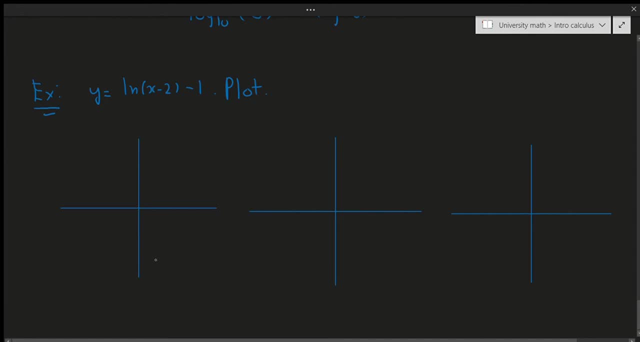 Okay, So let's start with the graph of ln of x. So ln of x is just going to look like this. Remember, it's the same as the normal logarithm. It just has bc. So it's going to look like the. 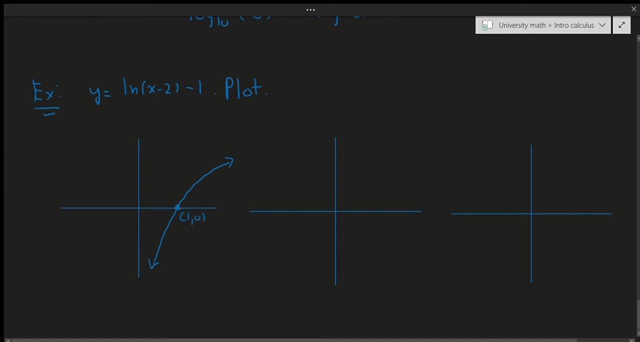 same. Okay, So that's going to be 1 comma 0 as the x-intercept, And then this one is going to be: y equals ln of x. The reason I know that this is 1 comma 0 is because in the exponential, 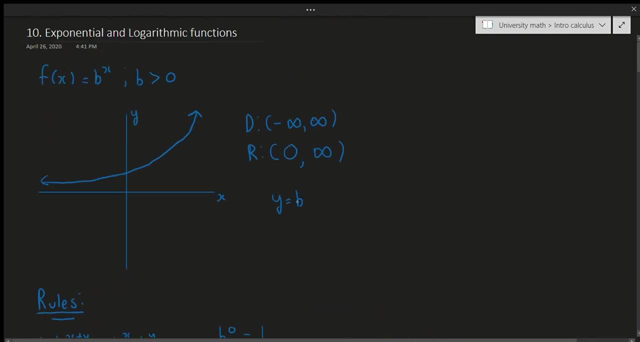 remember that the exponential is: y equals b to the x. So anything to the power of 0 is 1.. So b to the power of 0 equals 1.. So if I take the inverse, so if I get 0 comma 1 for the exponential, 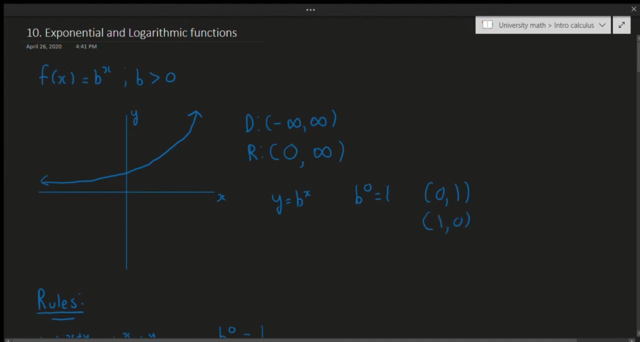 that means that when I take the inverse, I get 1 comma 0 for the x-intercept. So that's kind of why I knew that was the situation, Okay. So, with that being said, that's 1 comma 0.. 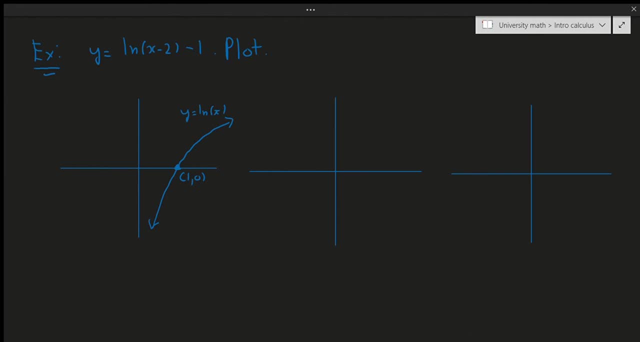 So now, if I go ahead and shift this to the right by 2 units, so that's this minus 2 here. Remember that the minus sign is the opposite of what do you do. So if it's minus 2, it just really means. 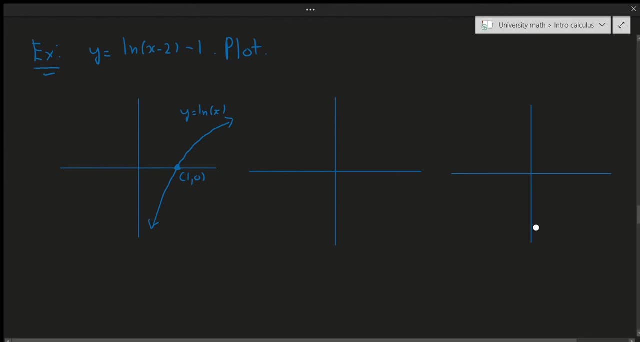 you go to the right by plus 2, not left. So remember that 0 is not defined. So 0 is an asymptote. So if I shift it to the right by 2 units, the asymptote shifts with it. So now the 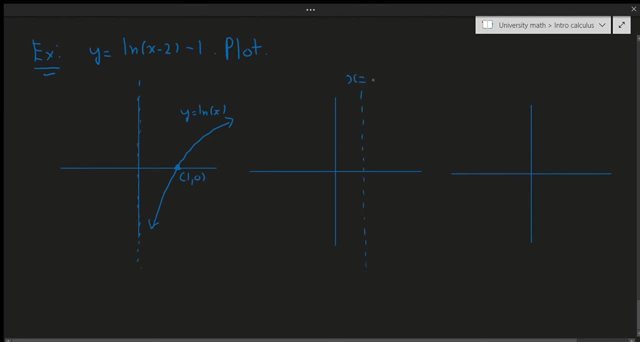 x equals 2.. And then this one right there, that's going to flip as well. So at this point right there, that's 3 comma 0. So this one is ln of x minus 2.. So nothing too wild. And then the last. 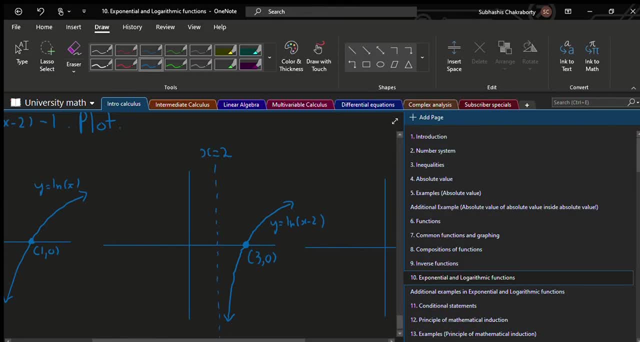 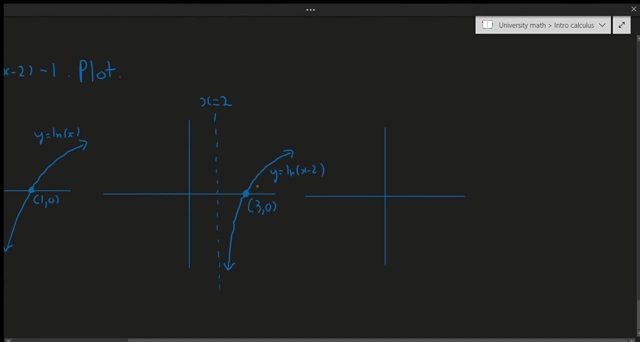 one. Oh, sorry about that. So the last one. we just have to do the same thing. So we just have to shift it down by 1 unit. So this point: 3 comma 0 becomes 3 comma minus 1.. So let me just keep. 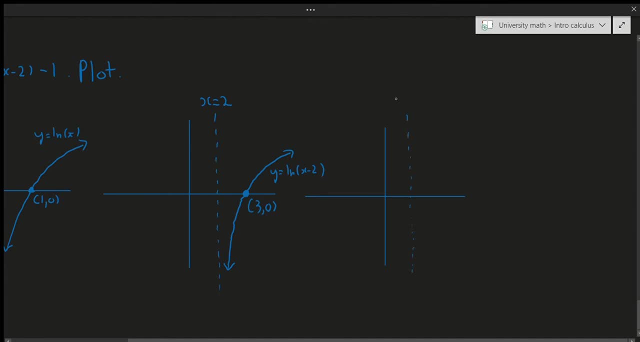 drawing the asymptote. The asymptote is not going to shift in any way, So that's still going to be x minus equals 2.. But now, this point right there, that point, right there, that's going to be 3 comma minus 1.. And now we finally have to graph: y equals ln of x minus 2 minus 1.. And that: